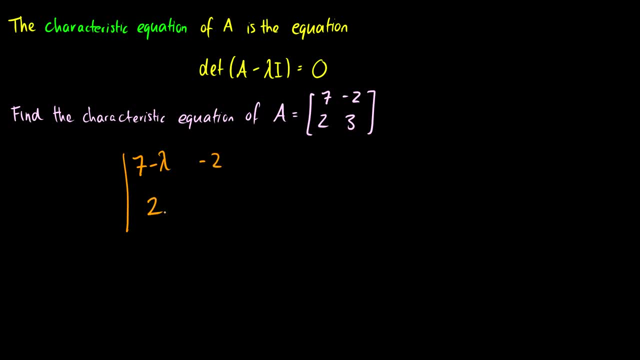 7 minus lambda, negative 2, 2 and this will be 3 minus lambda. Okay, so we want the determinant of this. Well, we know, this is just ad minus bc, so we're going to get 7 minus lambda, 3 minus lambda, minus lambda. 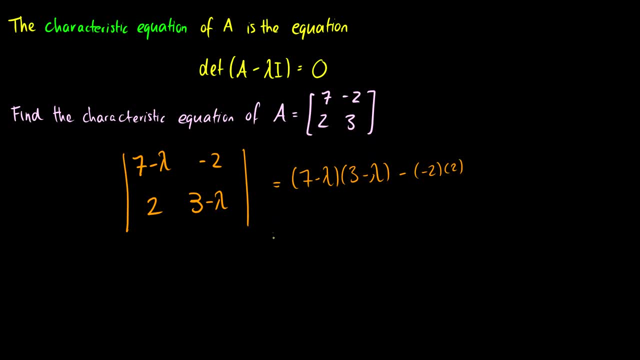 Minus negative, 2 times 2.. So we can expand this out. This is going to be 21 minus 10 lambda plus lambda squared. We're going to subtract negative 4, so we're going to add 4.. So if we rearrange this, this will be: 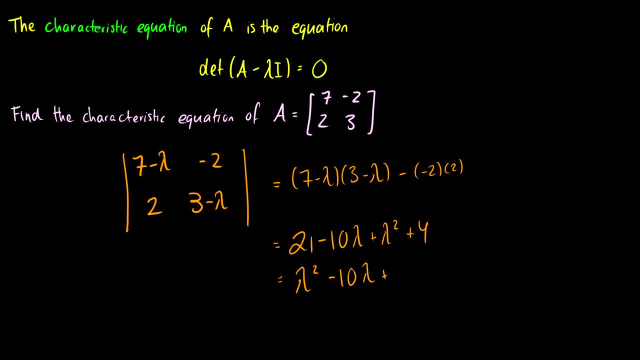 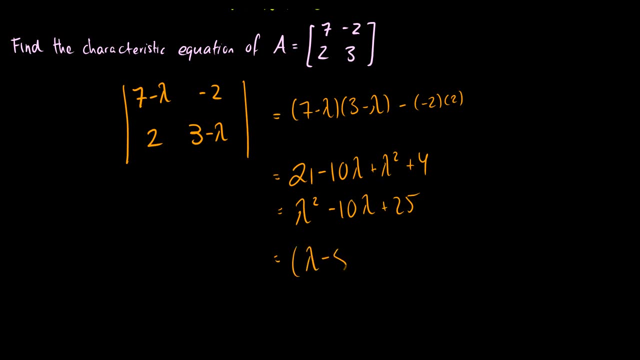 lambda squared minus 10, lambda plus 25, which is just going to be equal to lambda minus 5 squared. So we have our characteristic equation here. So what does this lead us to? Well, lambda minus 5 squared equals zero. So again we're finding the determinant equal to 0.. 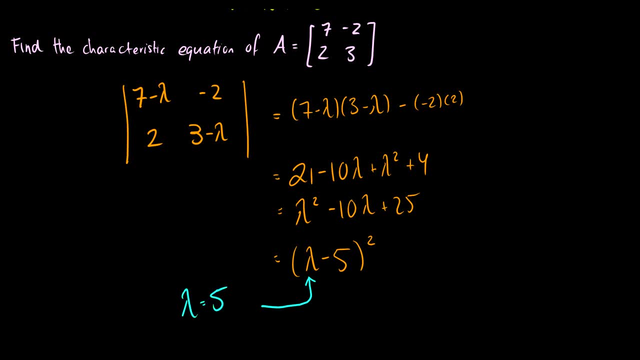 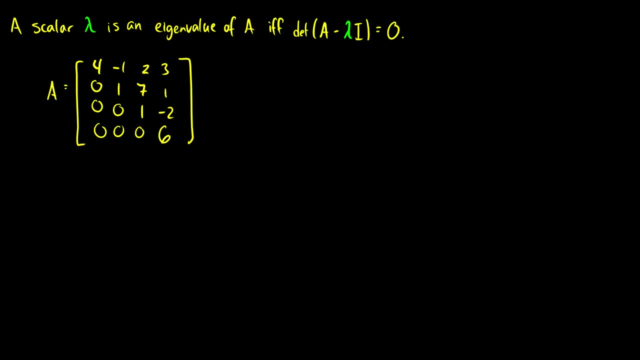 So what this means is that we have our lambda equal to 5.. So I wonder why we chose lambda for this variable. Well, let's take a look here. We say that a scalar lambda is an eigenvalue of a if the of a minus lambda i is equal to zero. So here I have a matrix in upper triangular form which is: 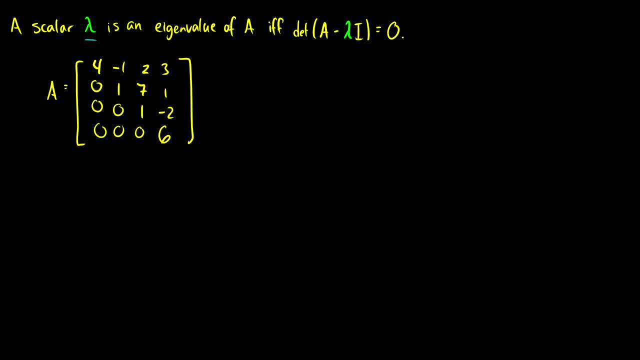 4, 1,, 1,, 6.. So we know that the eigenvalues of this matrix are going to be 4, 1,, 1, and 6.. So now I want to show that the determinant of a minus lambda. i will give us that, So it'll give. 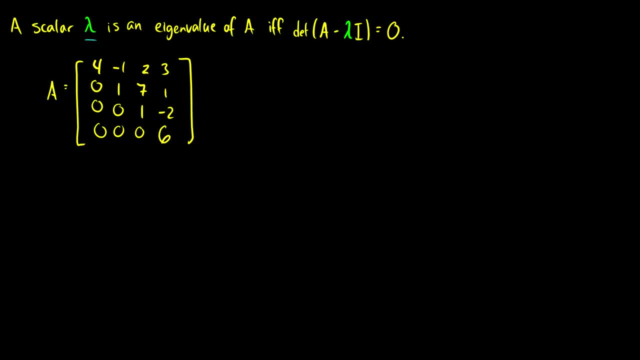 us lambda equal to 4,, 1,, 1, and 6.. Okay, so the determinant of a minus lambda i is going to be 4 minus lambda, negative, 1,, 2, and 3,, 1 minus lambda. this will be 1 minus lambda, 6 minus. 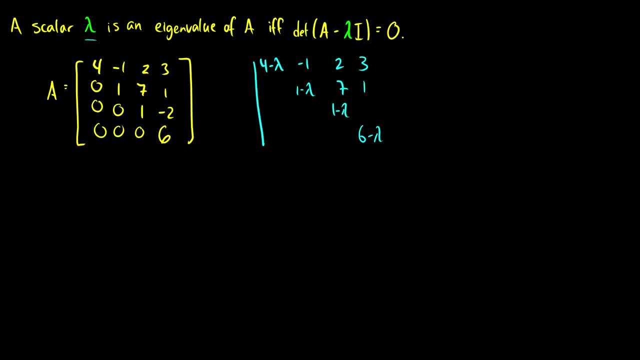 lambda, and then we're going to be left with 7,, 1, and negative 2.. The rest are zeros, So we can do some cofactor expansion here. So this is going to be 4 minus lambda and we're going to expand it. 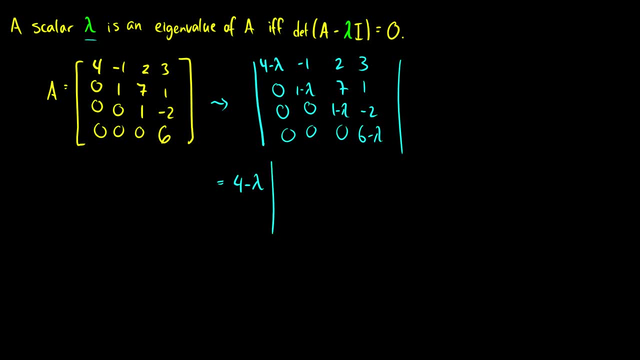 down the columns. So this will be multiplied by the determinant of 1 minus lambda, 7, 1, 0,, 1 minus lambda negative 2, and 0, 0, 6 minus lambda. So cofactor expansion. I'm just doing. 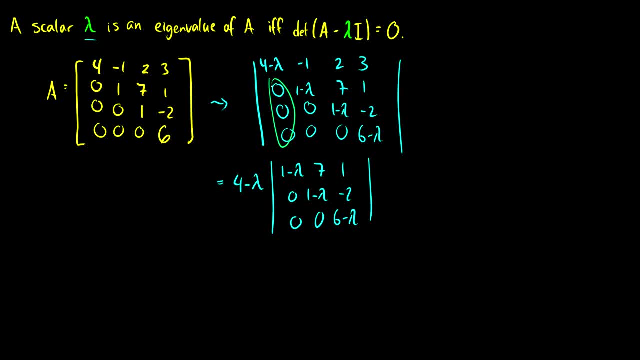 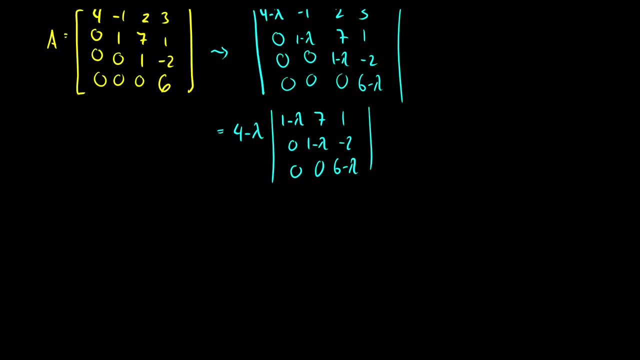 a shortcut here. So I know these are all going to be zeros, so I just took out the whole column And I was a little bit lazy with notation. but if you do this yourself and do a little bit slower, you'll see that this is the result that we get. Okay, so now let's do cofactor expansion across this column. 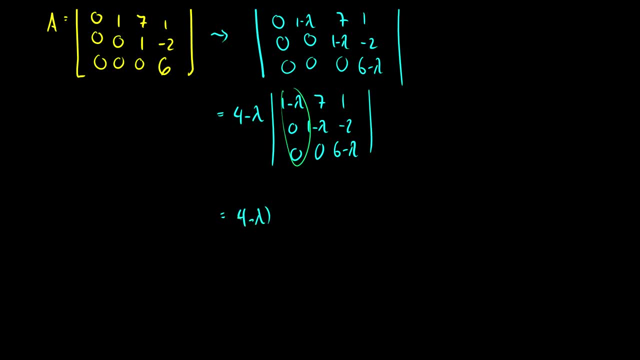 here. So we're going to get 4 minus lambda. multiplied by well, it's going to be 1 minus lambda times the determinant of 1 minus lambda, negative 2, 0, and 6 minus lambda. So we're going. 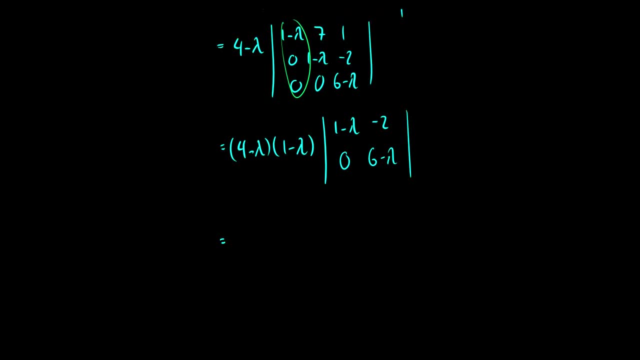 to get 4 minus lambda. So at this point we find the determinant of this 2 by 2 matrix. So it's going to be 4 minus lambda times 1 minus lambda. This will be 1 minus lambda times 6 minus lambda. 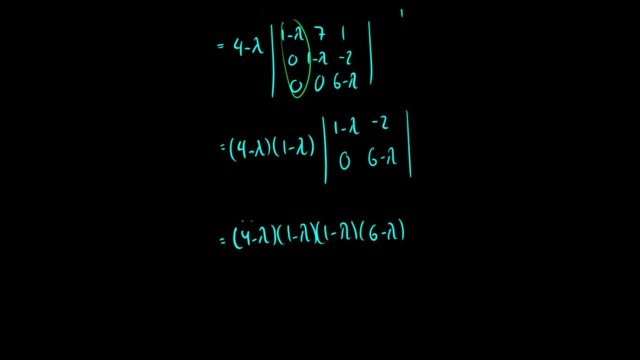 and then minus negative 2 times 0,, which is 0.. So we're left with 4 minus lambda times 1 minus lambda, squared times 6 minus lambda, which gives us the eigenvalue of 4 minus lambda times 1 minus. 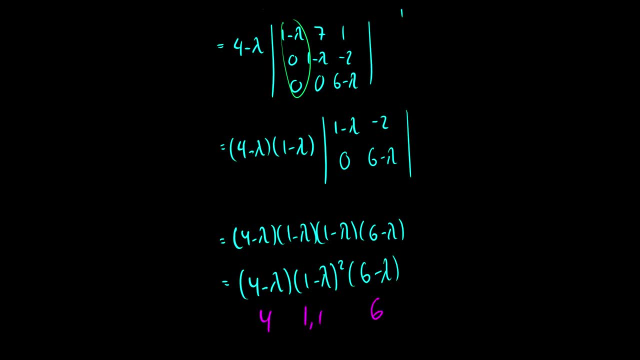 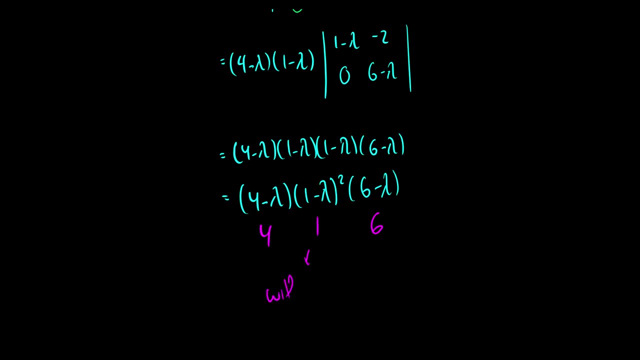 lambda squared. So this 1 minus lambda squared, really it just has the eigenvalue 1, but we say this is with multiplicity 2.. So this means that it appears as an eigenvalue twice, So it's multiplicity 2.. Okay, so that's how we find eigenvalues with determinants and characteristic. 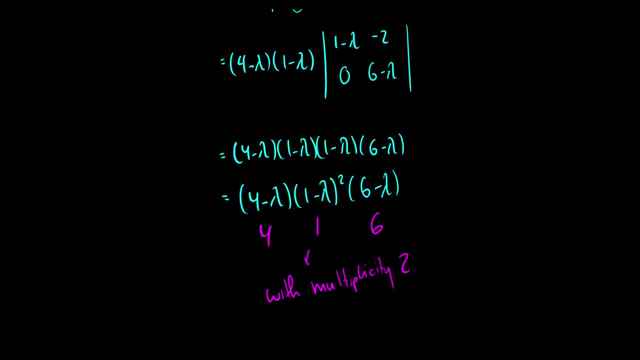 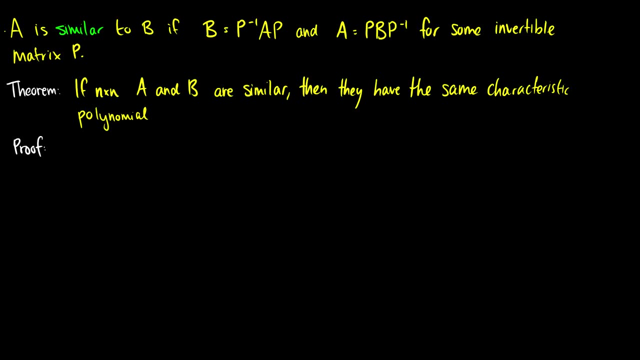 equations, So pretty straightforward. There's really not that much to it. So let's introduce something else really quick here, And this is important, because if we have two matrices, A and B, and they're similar, then they're going to have these same characteristic. 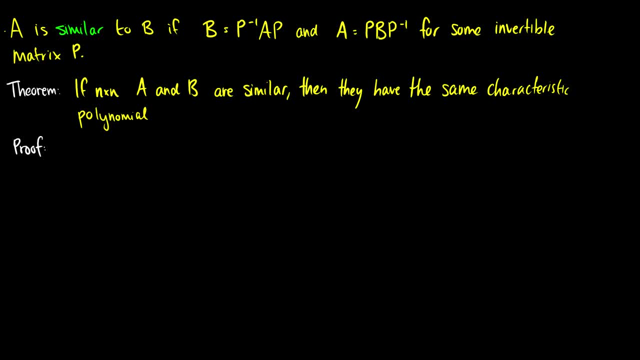 polynomials. So what does similar mean? Well, A is similar to B. if we can say: B is equal to P inverse, AP and A is equal to P, B, P inverse for some invertible matrix, P. This basically means that we can do a trigonometric equation. So we can do a trigonometric equation and we can do a. 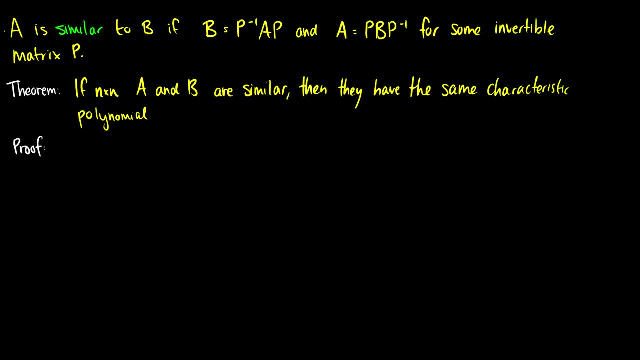 transformation on a vector B and we can do another transformation and then we'll get back to A. So they're similar in that sense. Okay, so if A and B are similar, then they have the same characteristic polynomial. So what are we really proving here? Well, we're proving that the 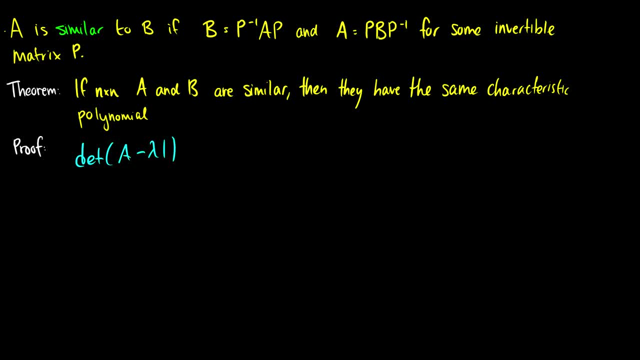 determinant of A minus lambda I is equal to the determinant of B minus lambda I. Okay, and that'll give us our eigenvalues Or, more importantly, our characteristic polynomial. So before we start working with determinants, I want to do some simplification first. So we have: A is similar to B, So we're assuming they're. 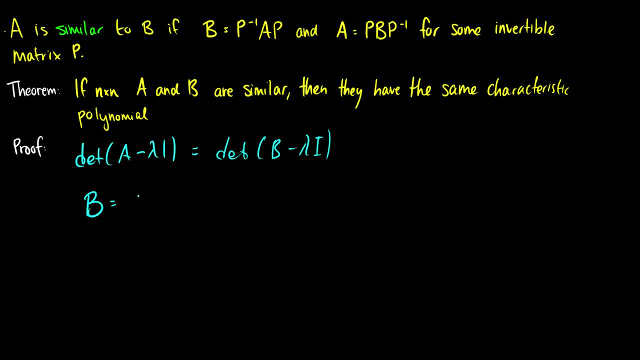 similar. So let's write B as P inverse times A times P. Okay, so then when we find B minus lambda I, really what we're finding here is P inverse AP, So B is equal to A plus B minus lambda I. So that's going to be a little bit easier to work with. 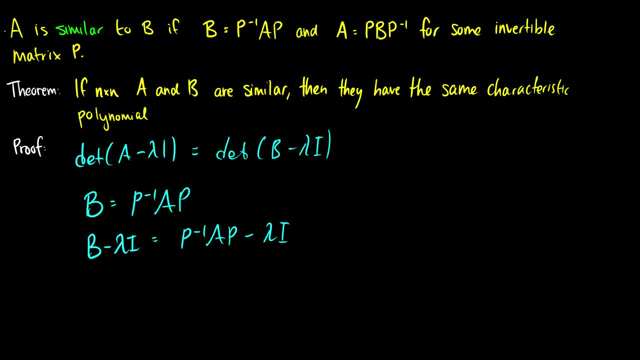 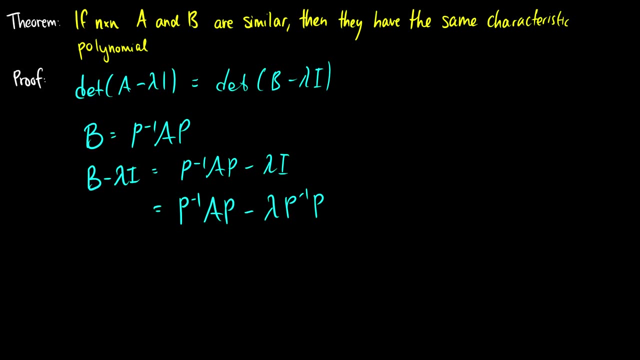 But well, if I want to factor some stuff out here, I can change I into P inverse P. So maybe that's better for factoring, because P is invertible. So P inverse P is going to be equal to I. So at this. 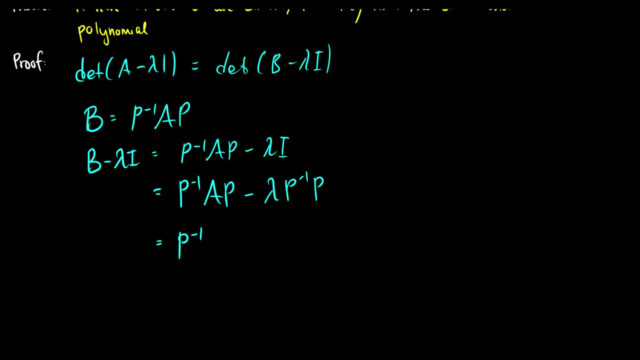 point. what we can do is we can factor out P inverse from the left, So that's P inverse times A, AP minus lambda P. and then we can factor out a P from the right side, so it's going to be P inverse times A minus lambda I times P inverse. Okay, so this is a nice start, because now I can. 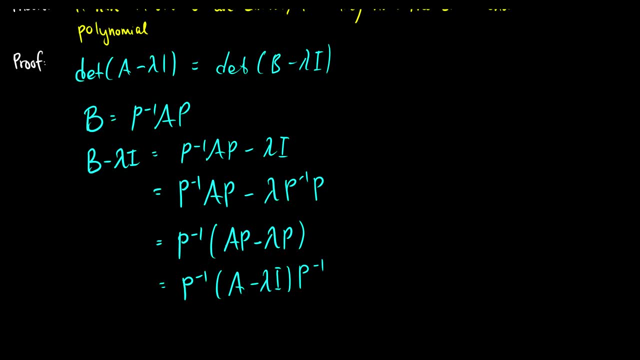 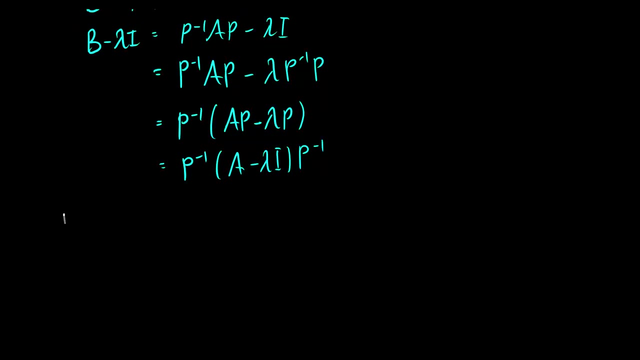 write B minus lambda I as P inverse times A minus lambda I times P inverse. So remember: here I want to show that the determinant of A minus lambda I is equal to the determinant of B minus lambda I. Okay, so we can write the determinant of B minus lambda I equal to the determinant. 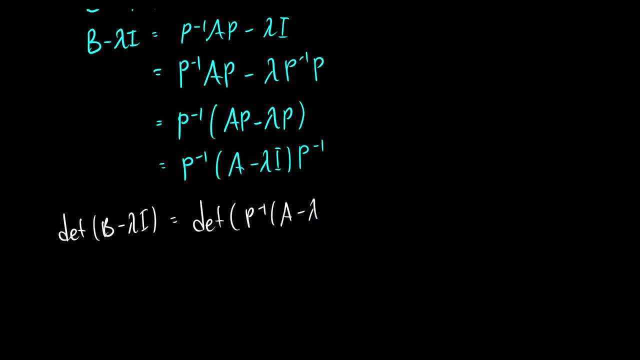 of P inverse times A minus lambda I times P. Okay, so what do we know about the determinant of matrices multiplied together? Well, we know that if we have A minus lambda I times P, we can write the determinant of B minus lambda I times P.